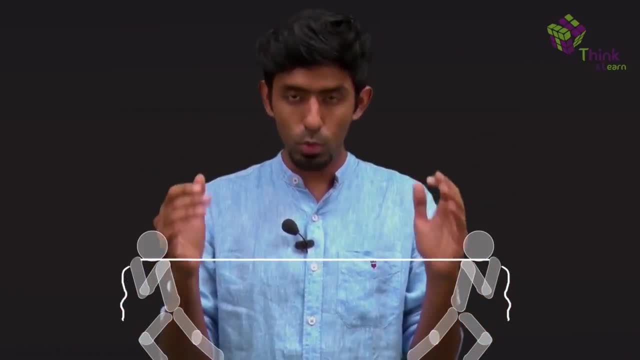 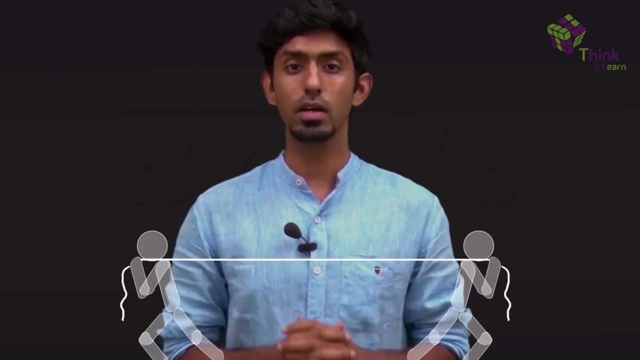 rubber band whose length increases and then comes back. But no matter what force you apply, we assume that the string is going to retain its length. We call it the law of conservation of string length, And whenever you see in a question the word inextensible string, what it means is: 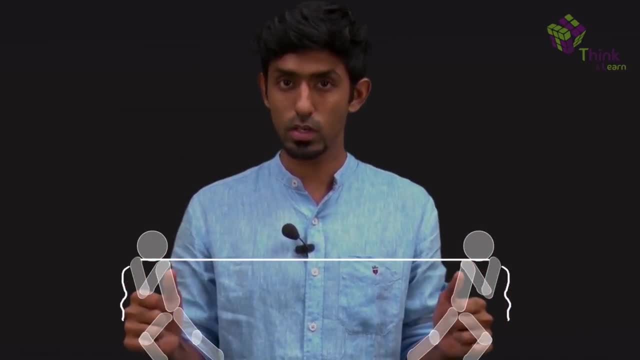 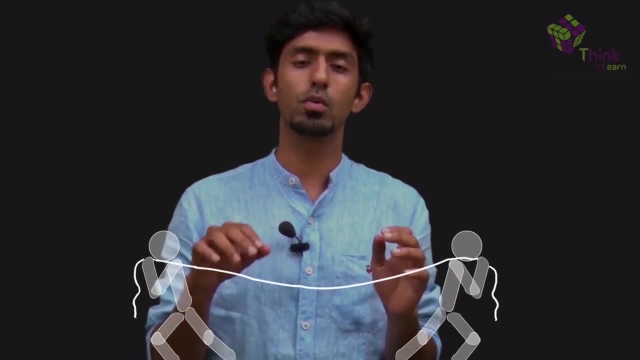 that this string's length in this direction will be a constant as long as it is tucked. The word t-a-u-t will mean that the string is not being pushed inside and becomes all what's called slack. So as long as you keep it in a straight line, its length is going to be a constant. 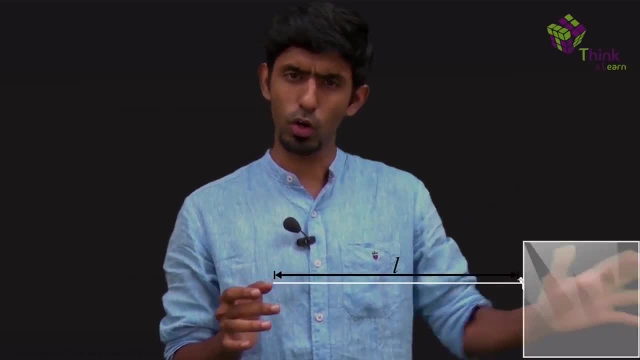 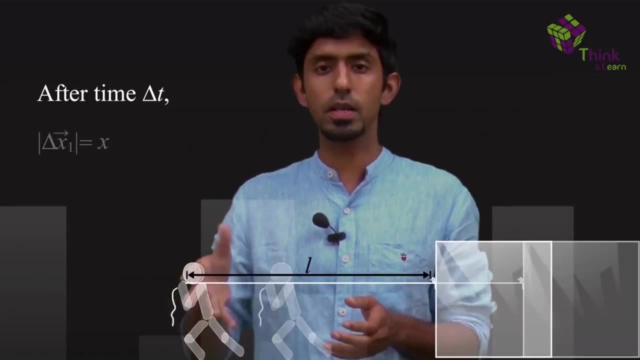 So if I take this inextensible string and attach one end of it to a block on a horizontal surface and I hold the other end and start walking after some time, let's say delta t, my displacement, let's say, is x, What will the displacement of the block be? 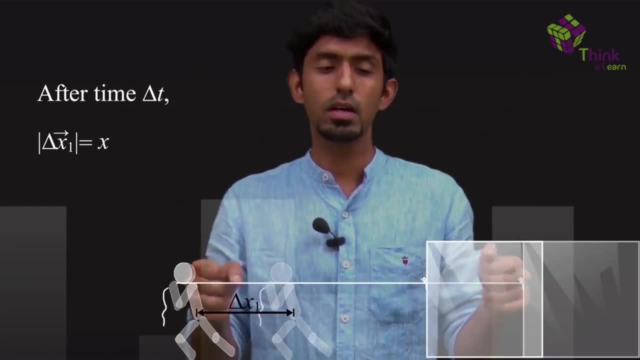 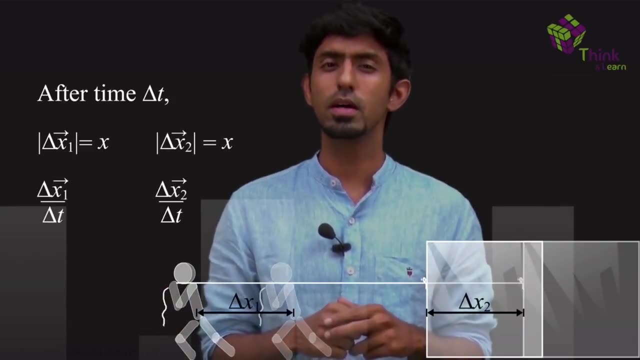 Because the string is taught and because it doesn't change its length. the displacement of the block must also be x. It seems clear from this picture. Now, if both of these took time, delta t, then the average velocities also must be the same for both. 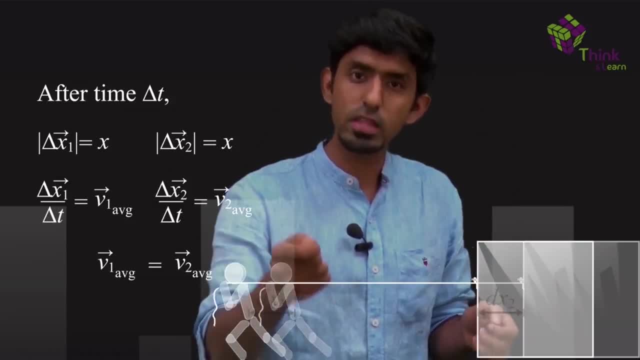 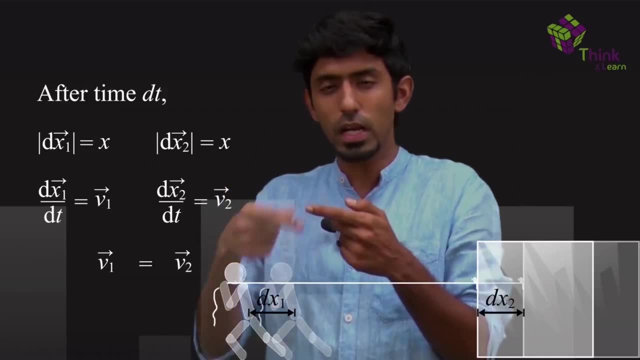 And you know that if I make this delta t really, really small, even then this relationship will hold, which means the instantaneous velocity must also be equal for both of them. Now, because I've started with delta t, I'm going to make this delta t equal for both of them Now because I've started 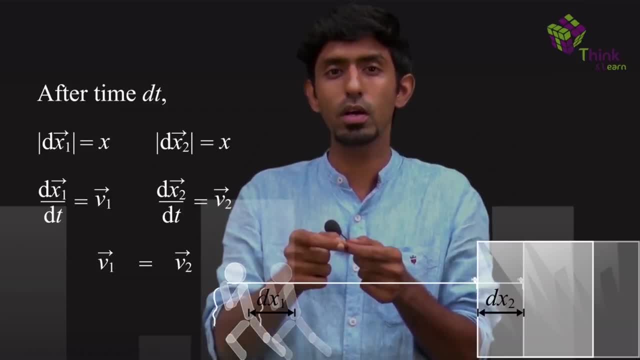 delta t. I'm going to make this delta t equal for both of them Now, because I've started with with displacement and given an argument for velocity, I can do something very symmetric for going from velocity to acceleration. So this must imply that their accelerations must also be equal. 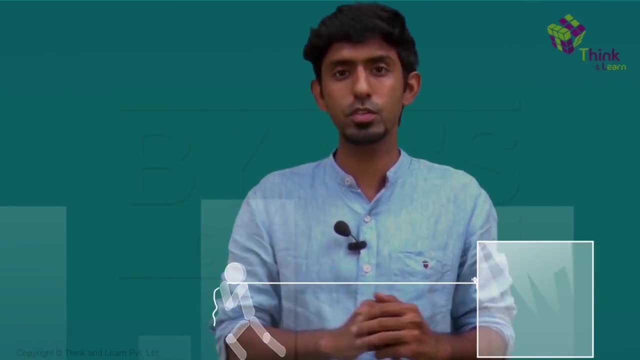 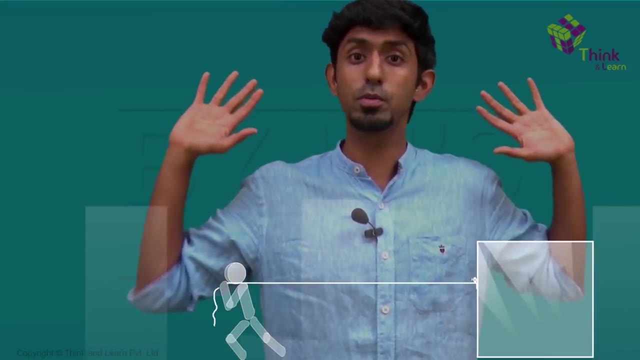 If this argument seems a little long, let's take another one. Let's move into the frame of reference of that man. What will he see? He turns back and looks at the block. Throughout his journey, he will see the block being at rest from his point of view. And if this must be true, 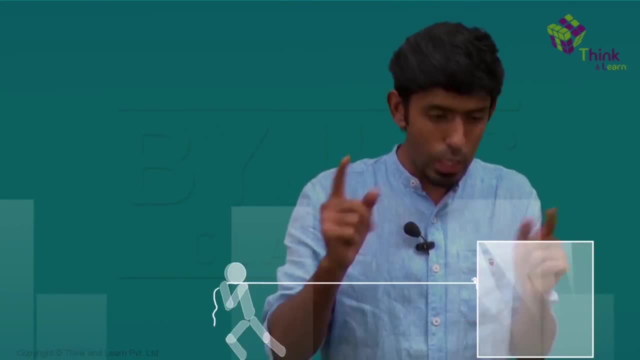 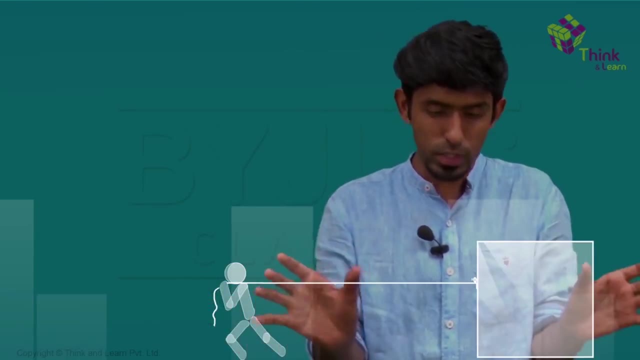 every variable- displacement, velocity, acceleration- all of this must be equal for both of them, Otherwise this would not happen. So both these arguments you can use to show that in such a scenario, where two objects are connected by an inextensible string and the movement happens in a direction where the string is taught, 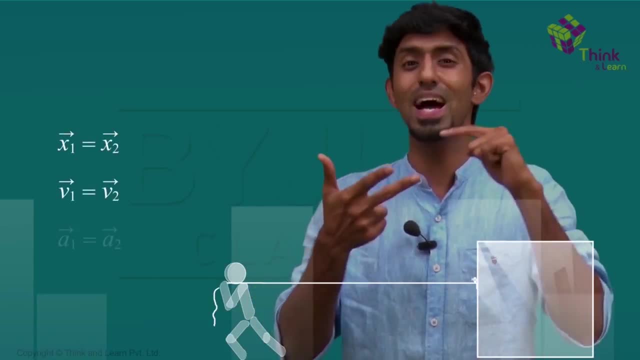 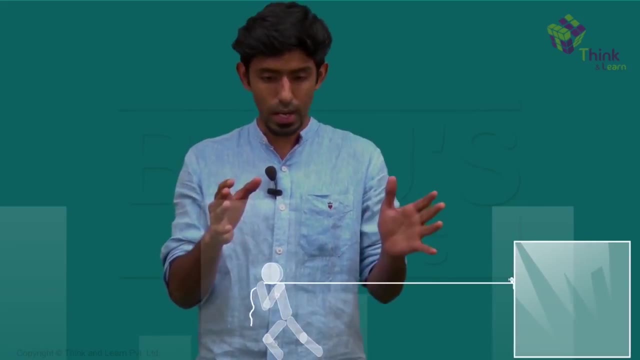 the two bodies must have the same displacement, the same velocities and the same accelerations. Now imagine that this man is pulling that block, dragging it along with him and moving such that both of them have an acceleration of a. Now you know, one of them has a.